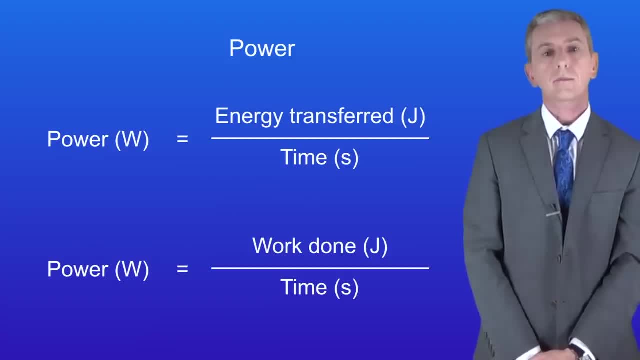 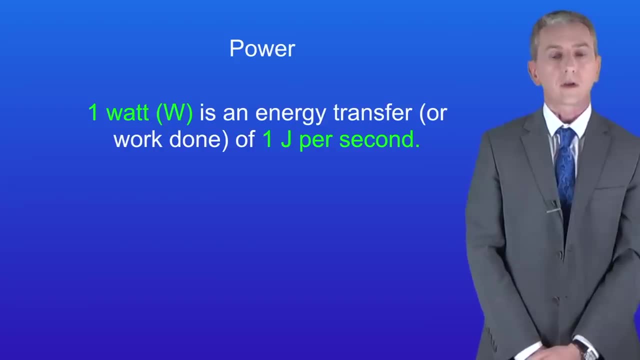 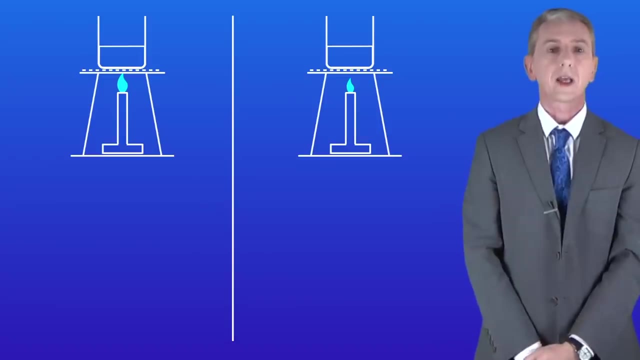 in joules divided by the time, in seconds. Now the unit for power is the watt, and that has a symbol, capital: W. One watt is an energy transfer or work done of one joule per second. I'm showing you here two beakers containing the same volume of water. Both of these are being heated by Bunsen. 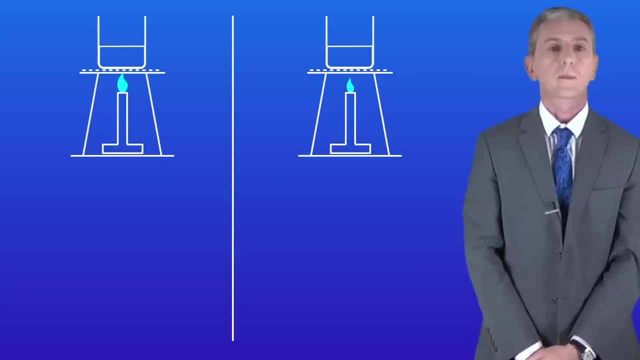 burners and we're going to calculate the power of these energy transfers. The left hand Bunsen burner is transferring a total of two hundred and fifty thousand Joules per second After the of thermal energy in 500 seconds, and the right hand Bunsen burner is transferring a total of 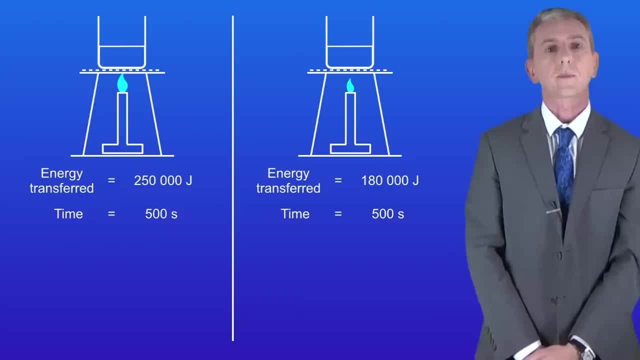 180 000 joules of thermal energy in 500 seconds. The power is the energy transfer divided by the time. so if we look at the left hand Bunsen burner, we can see that we've transferred 250 000 joules of thermal energy in 500 seconds. Putting these numbers into the equation gives us a power of 500. 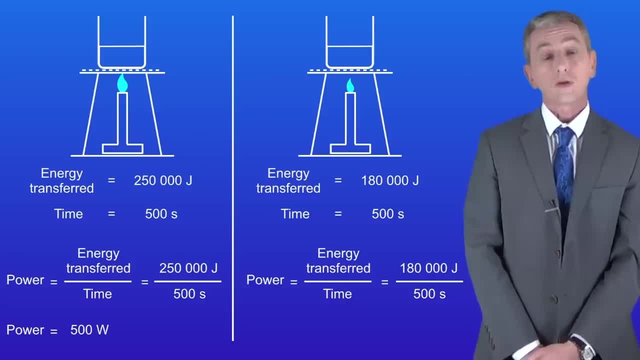 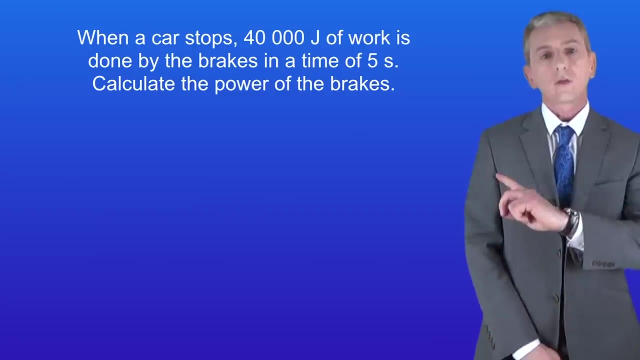 watts. Looking at the right hand Bunsen burner, we're transferring 180 000 joules of thermal energy in 500 seconds. Putting these numbers into the equation gives us a power of 360 watts. So, as you can see, calculating power is relatively straightforward. Here's a question for you. 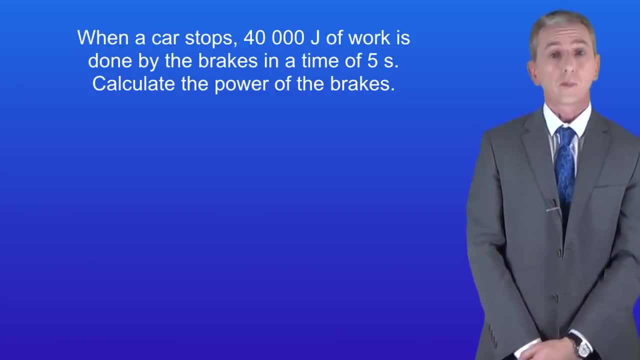 When a car stops, 40 000 joules of work is done by the brakes in a time of five seconds. Calculate the power of the brakes. Pause the video now and try this yourself. Okay, here's the equation that we need to use. Power equals work done in joules divided by the. 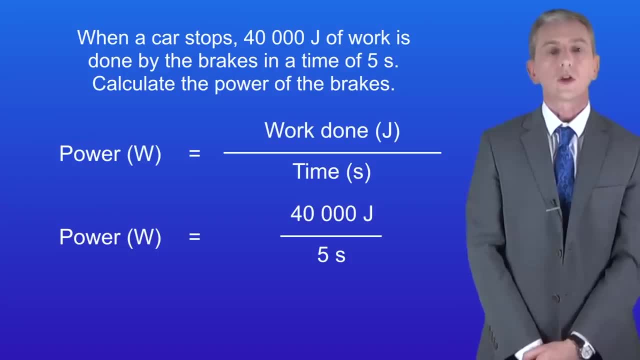 time in seconds. So the work done is 40 000 joules and the time is 5 seconds. Dividing 40 000 by 5 gives us a power of 8 000 watts, and that's our final answer. Here's another question for you to try. I'm showing you here two motors lifting two identical 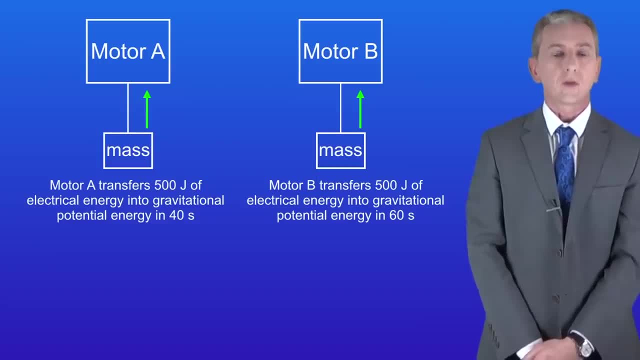 masses. Motor A transfers 500 joules of electrical energy into gravitational potential energy in 40 seconds. Motor B also transfers 500 joules of energy, but this motor takes 60 seconds. Calculate the power of both motors. So pause the video and try this question yourself.